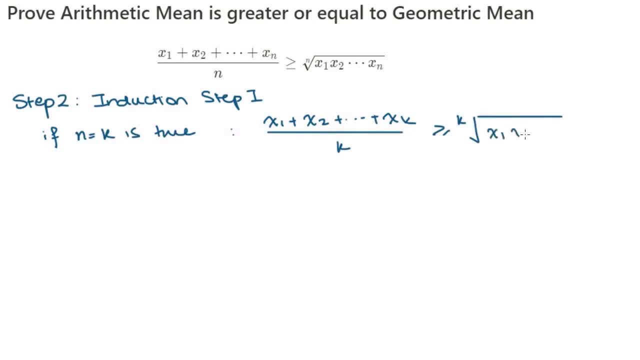 k all over k is greater than or equal to the kth root of x1, x2, dot, dot, xk, then we want to prove that n is equal to 2k. is true x1 plus x2 plus all the way up to x2k, all over 2k, because there. 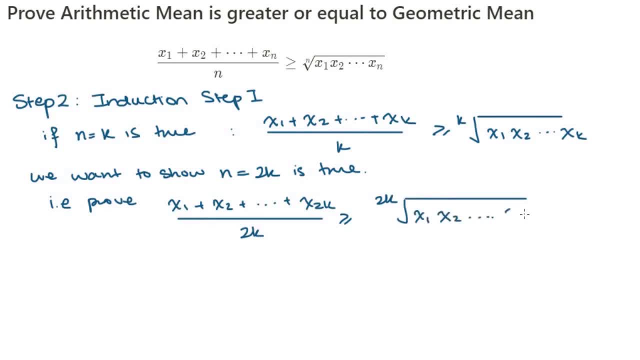 are 2k terms is equal to the 2kth root: x1, x2, dot, dot, x2k. that's our hypothesis and the top line is our star. let's try to substitute our star equation into the hypothesis. so the left hand side of the hypothesis is x1 plus x2, all the way up to x2k, over 2k, which we can rewrite by splitting. 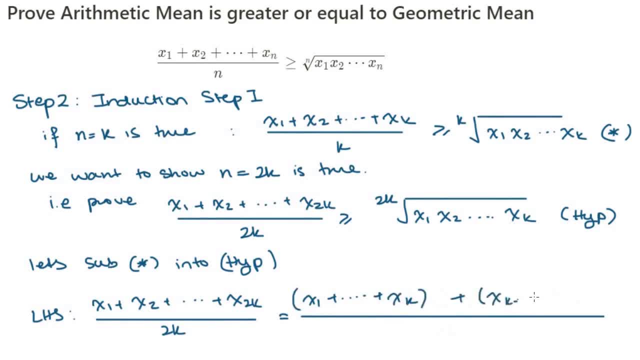 up the, the top half of the fraction, into x to xk and x? k plus 1 to x2k. the first part of the equation we can rewrite as k times the kth root of x1 all the way up to xk, and the second part of the equation is k times kth root of xk plus 1 all the way up to x2k. 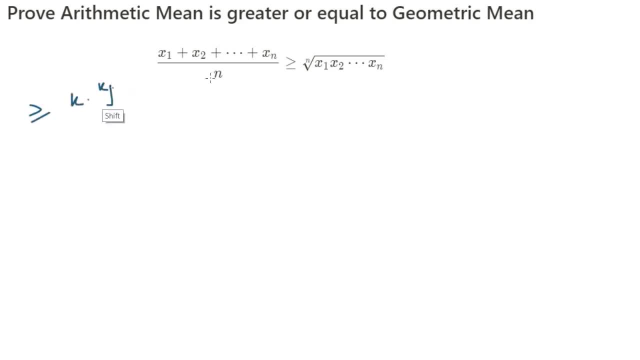 so the left hand side of the hypothesis is going to be greater than or equal to k times the kth root of x1, x2 dot dot xk plus k times the kth root of x, k plus 1, x k plus 2 dot dot dot x2k. 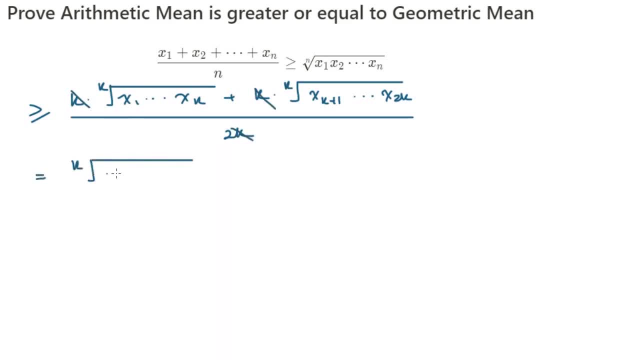 all over 2k. cancelling out the k's, we get the kth root of x1- x2 k plus 1 x k plus 2 dot dot x2k. x1, x2 dot dot xk plus the kth root of xk plus 1 xk plus 2 dot dot dot x2k, all over 2.. And we 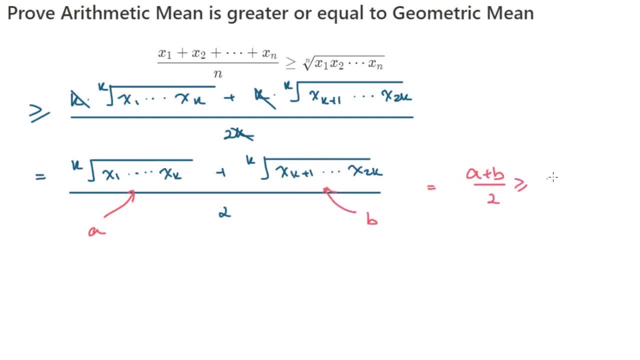 notice. this is of the form: a plus b on 2 is greater than or equal to root ab, with just two terms, which we've established is true from our initial case. Therefore, the left hand side of the hypothesis is greater than or equal to the square root of the kth root of x1, x2, dot, dot, xk. 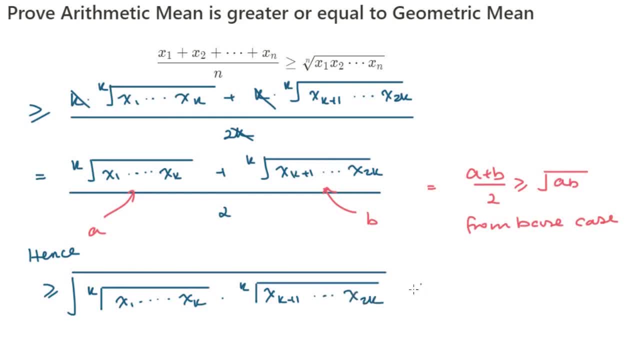 times the kth root of xk plus 1 xk plus 2 dot dot x2k, which is equal to the 2kth root of x1, x2 dot dot xk times xk plus 1 xk plus 2 dot dot x2k. Therefore, if n is equal to k is true, then n is. 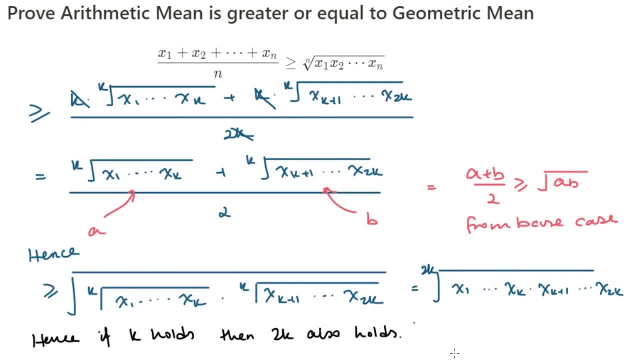 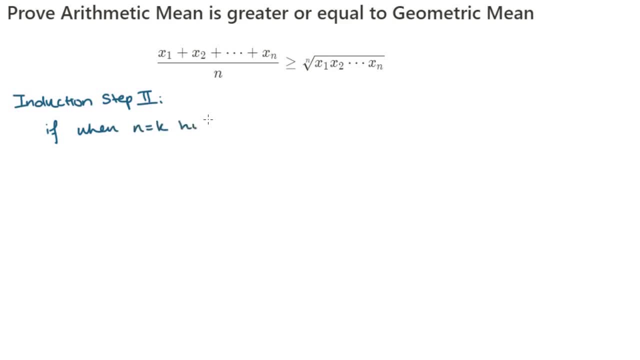 equal to 2k is also true. That was the forward step of our induction. Now on to the backward step. When n is equal to k is true, we want to show that n is equal to k minus 1 is also true. The assumption is that x1 plus x2 plus. 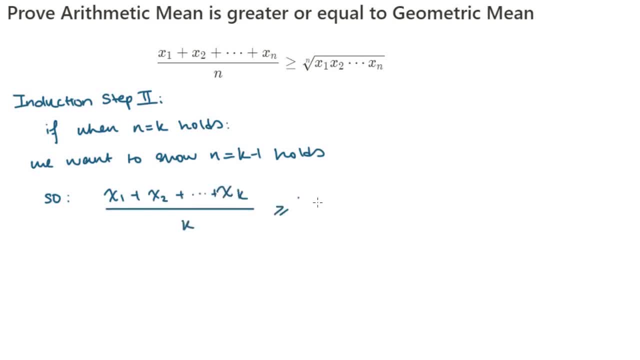 dot, dot, dot all the way up to xk. over k is greater than or equal to the kth root of x1, x2, etc. xk. This is true for all xk. So what if we let xk be a very specific term and this term is x1 plus x2 plus all? the way up to xk minus 1, xk plus 2, dot dot xk. So what if we let xk be a very specific term, and this time is x1 plus x2 plus all the way up to xk minus 1, xk minus 2 plus all the way up to xk minus 1. 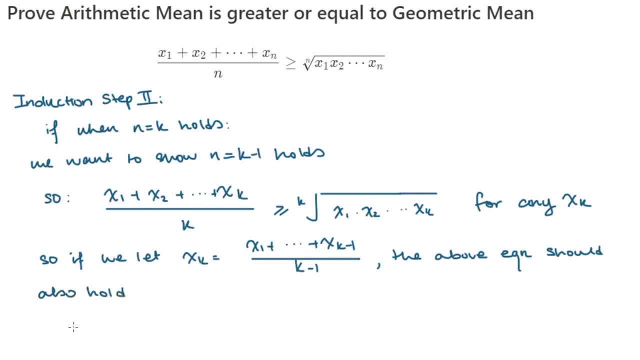 over k minus 1. so if we let x k be this very specific term, the above equation should also hold. let's substitute: x k is equal to x 1 plus x 2 plus plus x k minus 1 over k minus 1 into the left hand. 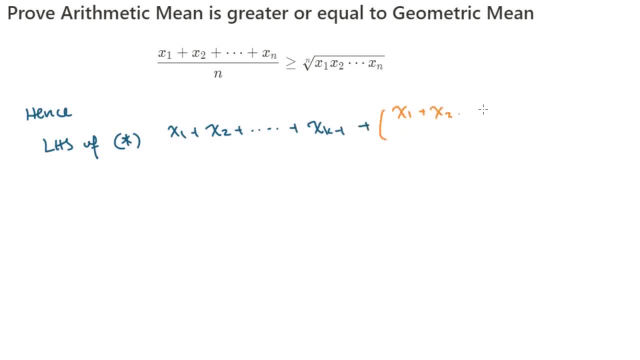 side of the star. our assumption as follows. you can see the substitution for x k in orange. something really magical happens. when you expand the fraction and collect like terms, you get this cancelling out the k's. you end up with x 1 plus x 2 plus all the way up to x k minus 1 over k minus 1. 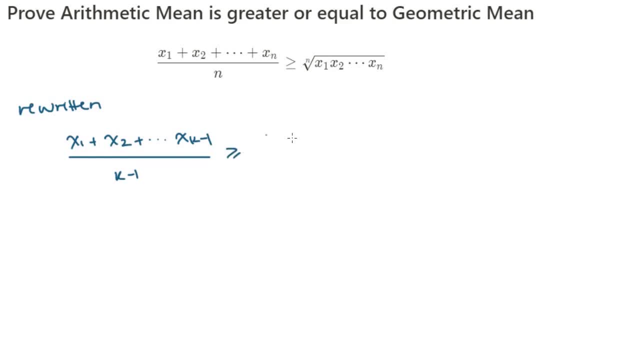 so let's rewrite it and let's substitute: x is equal to x 1 plus x 2 plus all the way up to x k minus 1, over k minus 1 into the right hand side as well, and raise both left hand sides and right hand side to the power of k, like so. 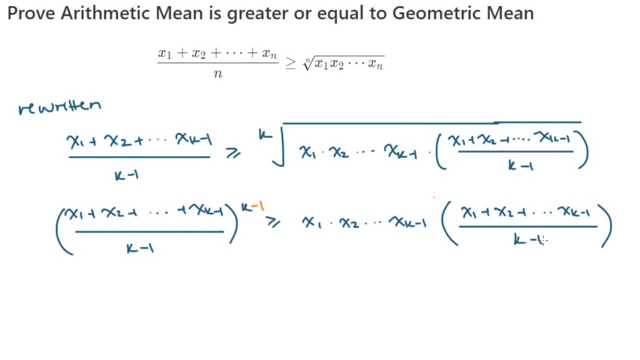 divide both sides by the brackets within the brackets, and we can do this without changing the sign, because we know what's in the brackets is definitely positive because each term is non-negative. once we take the k minus 1th root of both sides, we see that 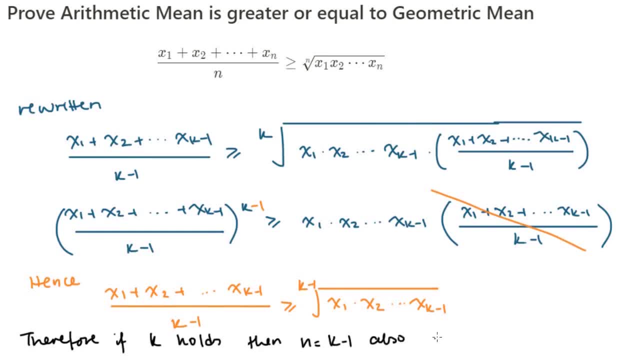